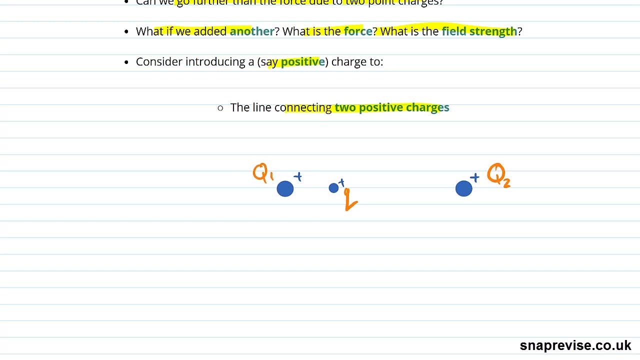 that Q1 and Q2 are experiencing. we just care what forces this one's experiencing. So we know it's going to experience a force- we'll say F1, that pushes it away from this Q1, because it's being repelled by that one. so we'll call that F1.. But it's also going to experience a force F2,. 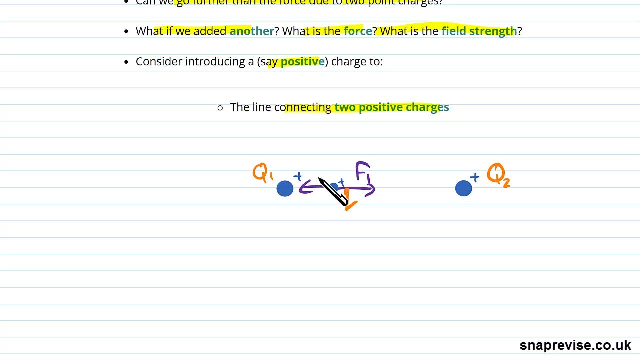 which is going to go in the opposite direction. right, It's going to experience a force F2 like this: away from this particle here, because this particle is also positively going to repel this smaller charge in the opposite direction. So we're going to do a little bit more of that. 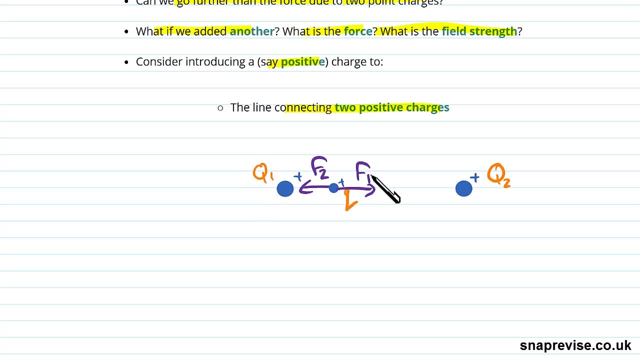 direction towards Q1. And so the net force is going to be kind of the difference of these two. So what do we need to do? Let's first just write down that our resultant force F- we'll call that F- net is going to be- well, it's going to depend. we can really see here which direction it's going. 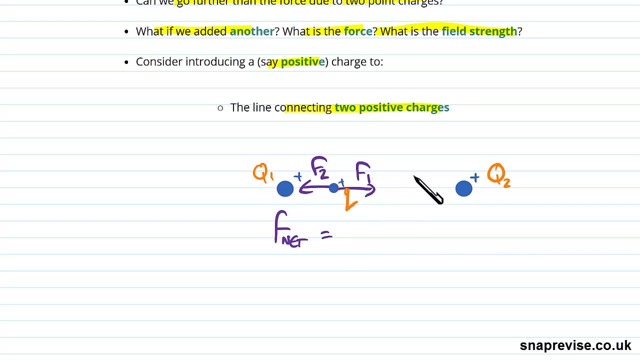 to end up going in just depends which one's you know stronger out of F1 and F2.. And so we can just perhaps assume fairly that F1 is going to be bigger than F2, just because you know, because it's closer to Q1 than it is to Q2.. Maybe Q1 and Q2 are similar. It could end up being the 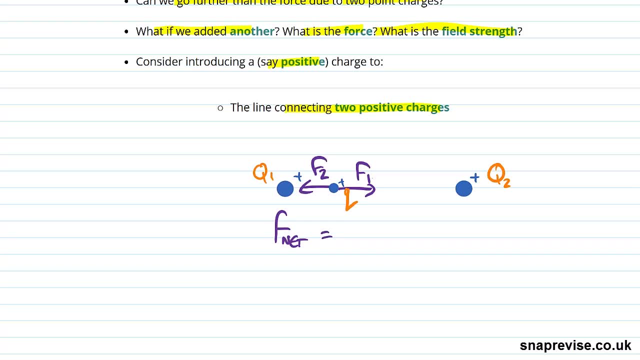 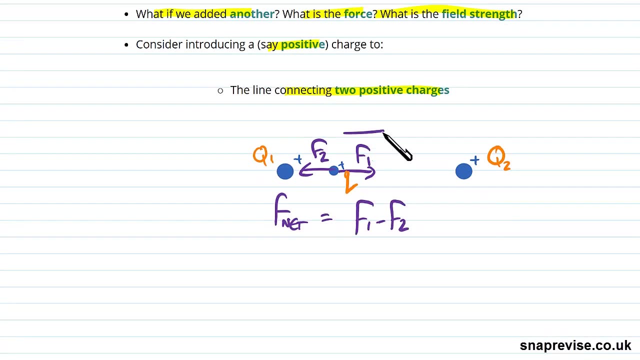 other way. It's not too important. It's just going to affect the sign of F net, nothing else. So we'll just say it's F1 minus F2. And we're going to assume that it's going to be in this. 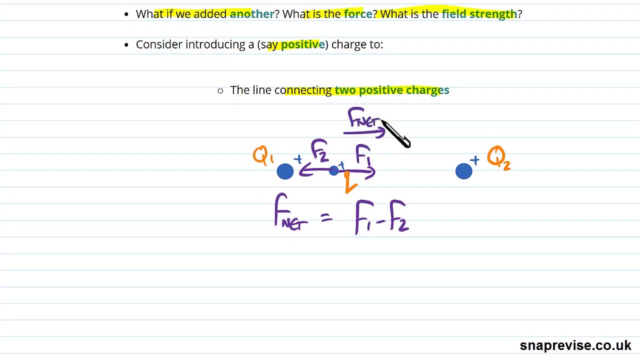 direction, overall F net. But again, that stuff is all. it doesn't affect the working here, It just affects. you know, in the end of this. with negative then we just mean that actually we'd be going in this direction but we'd calculate the magnitude correctly. So that's the first thing. 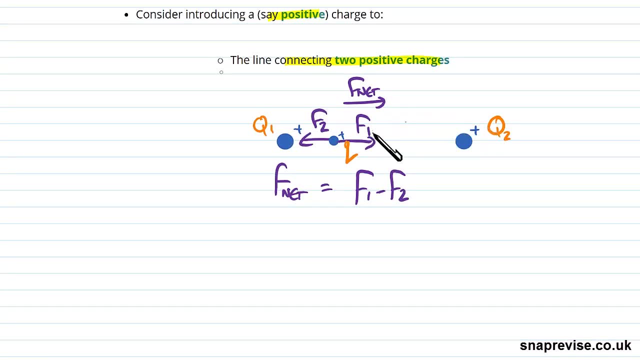 And then we just need to say: well, what is F1 individually? And that is where we basically think about the Coulomb's law set up, but where we've just got these particles and we ignore this one, So we can imagine that one's not there. So what's that going to be? Well, if we're interested, 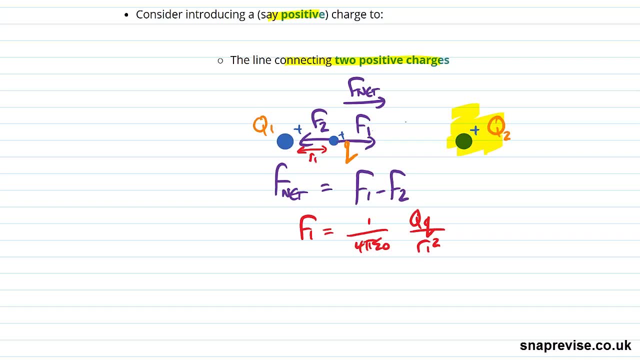 that's going to be. F1 is just going to be 1 over 4 pi, epsilon 0, capital, sorry, Q1, Q over R1, squared where R was the distance there, And equally we could do the same thing for you know. 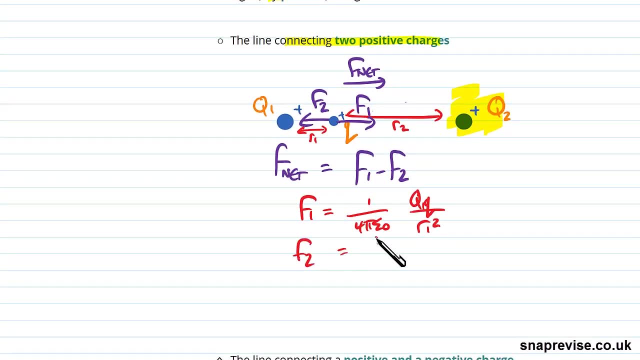 R2 for this distance and say that our second force is going to be exactly the same thing, just with a, with an Q2 in there and an R2 there instead. But really we don't care about this bit too much.